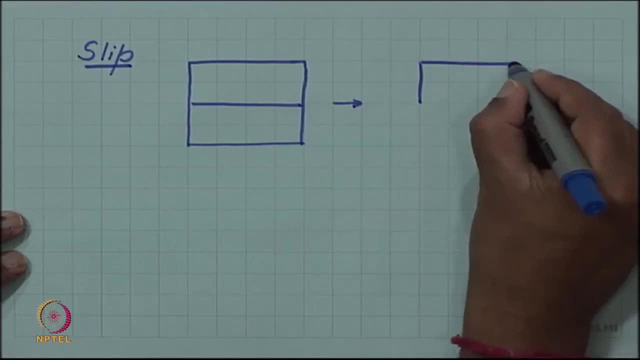 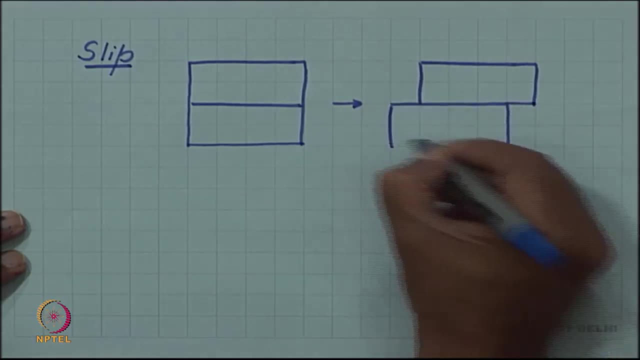 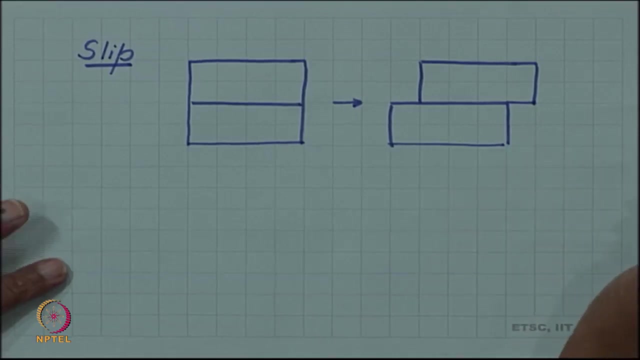 So we have seen this model of plastic deformation: that one half of the crystal slides over the other half on a slip plane in the slip direction. However, what they realized, the proposal, the new proposal, was that this sliding need not happen in one go. it may happen that one side of the crystal has slide whereas the other side has. 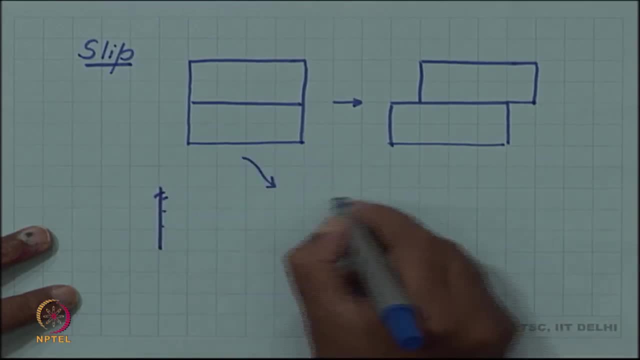 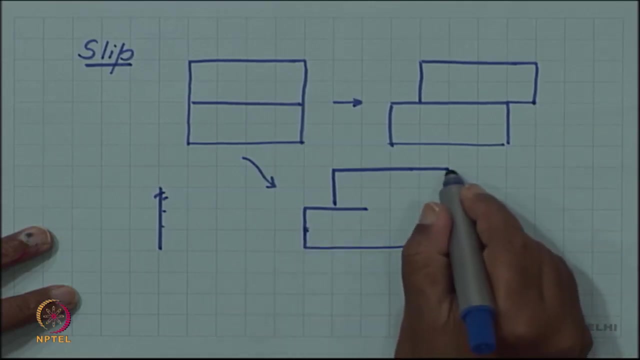 not slide, So may be in the intermediate stage the deformation is something like this. So this is also the deformation of the crystal. There is no deformation of the crystal, but there is no deformation of the crystal. So we can easily solve this problem. 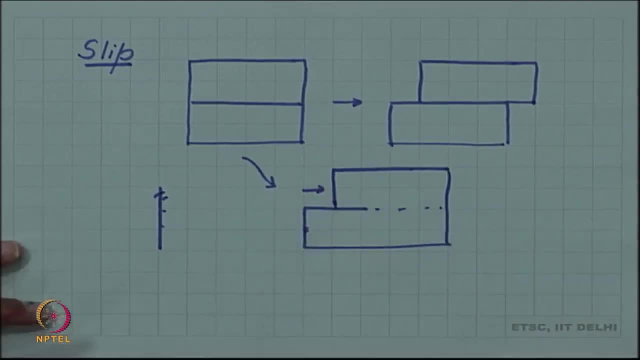 So if I look at this plane, on this plane up to some point, up to some point sliding has happened. So on the left side I have this step, but on the right side I do not have this step. This is possible because the entire crystal is not really a continuum rigid body, but 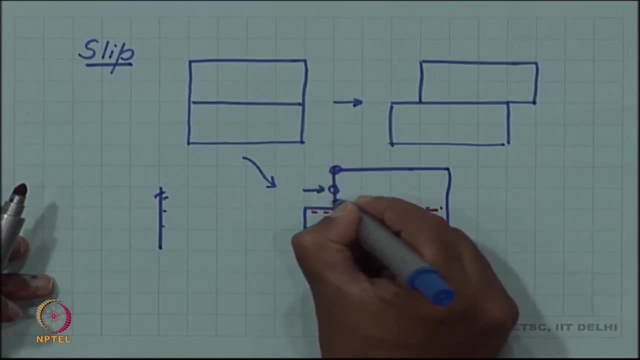 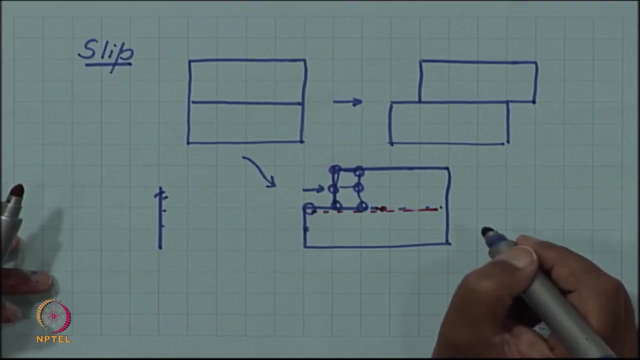 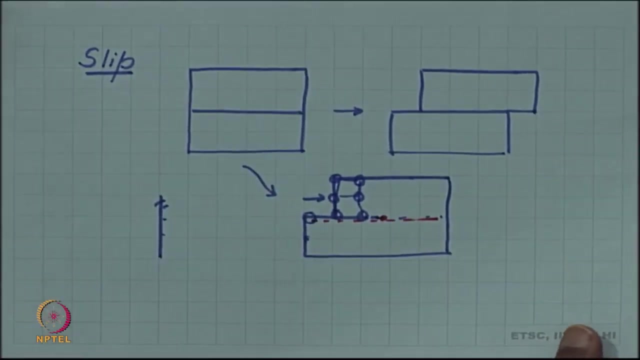 is made up of atoms and it is possible for atoms and the atomic bonds to distort and deform in a way that sliding happens on one part but the other part has not yet fled. So this was the proposal. So, essentially, what is being proposed is: 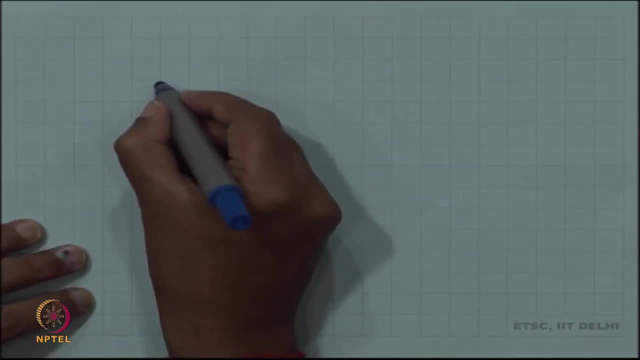 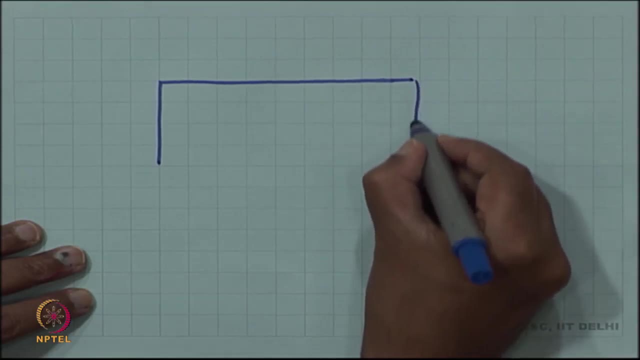 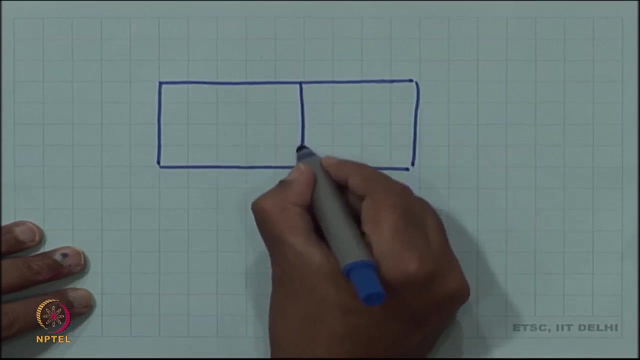 So this was the proposal. So, essentially, what is being proposed is That on the slip plane, if you think of the slip plane, slip has not taken place over the entire slip plane, but part of the slip plane has slipped and on the other part there 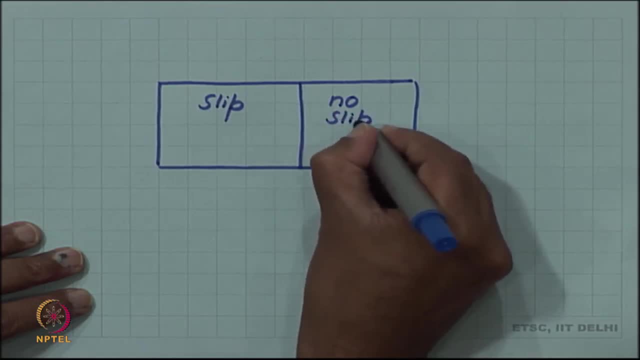 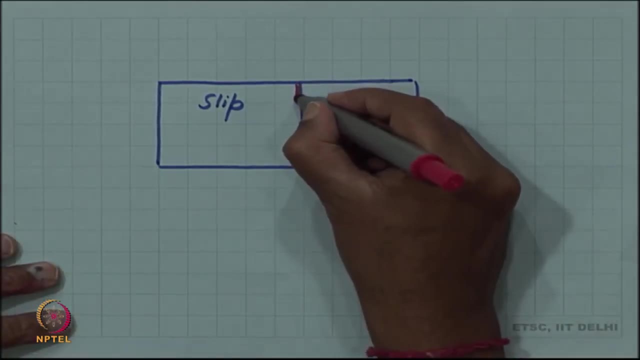 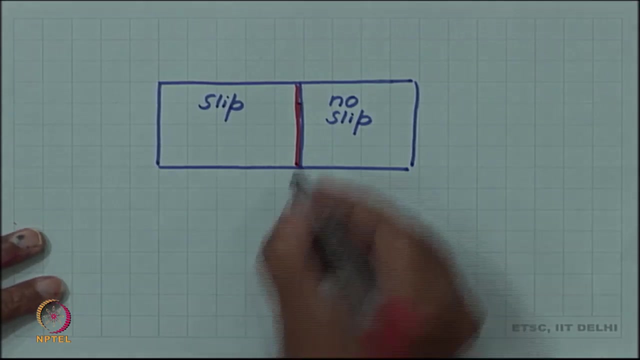 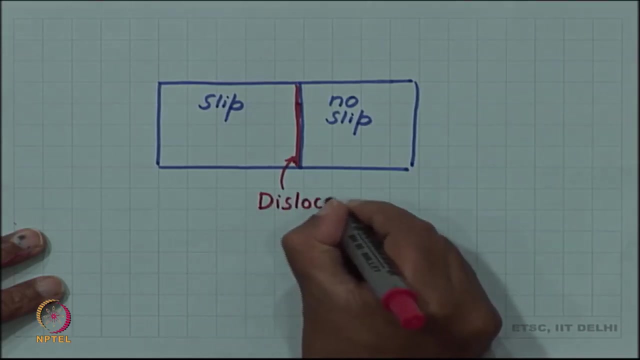 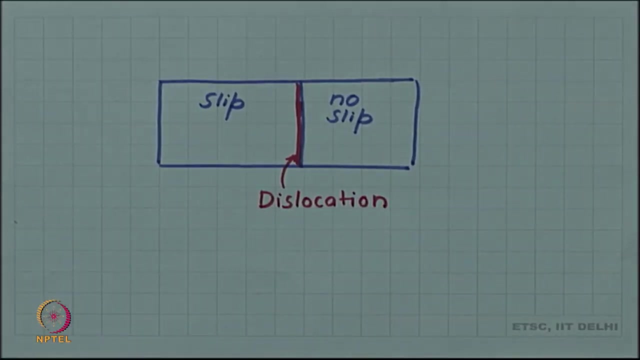 is no slip And, if you recall from your defect chapter, this was what we considered As a dislocation line. So what is really being proposed? that a dislocation is present during deformation, a boundary between slip and not slip plane we called dislocation. but why should dislocation lead? 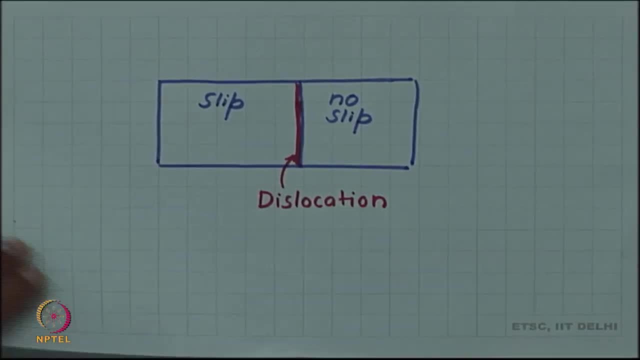 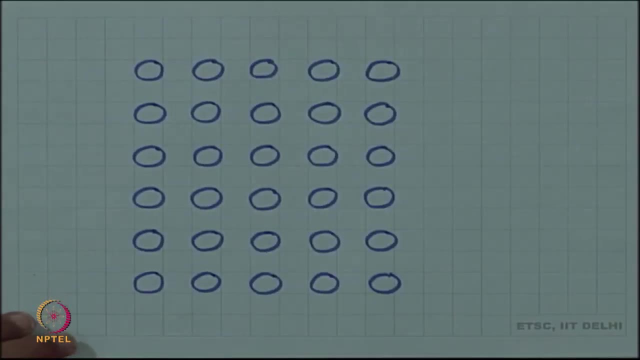 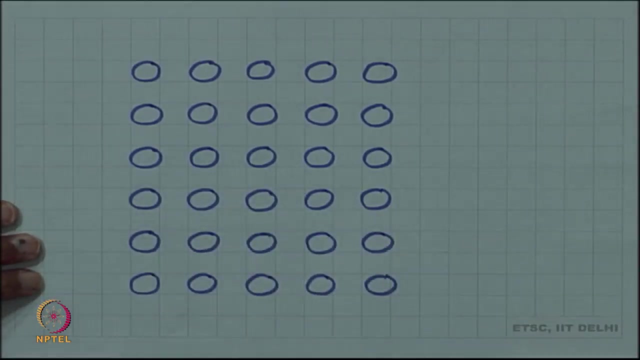 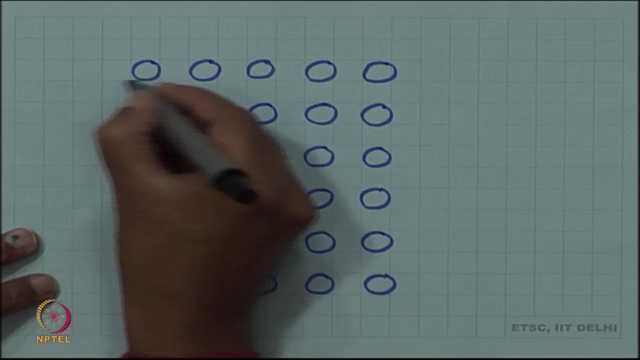 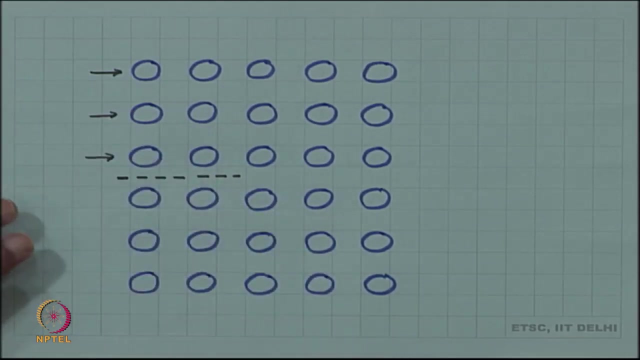 to a easy deformation of the material. So let us look at that in this picture. So suppose this is a crystal and suppose we cut this crystal on some slip plane and after this cut I try to push this upper half above the slip plane with respect to the lower half and suppose I have made. 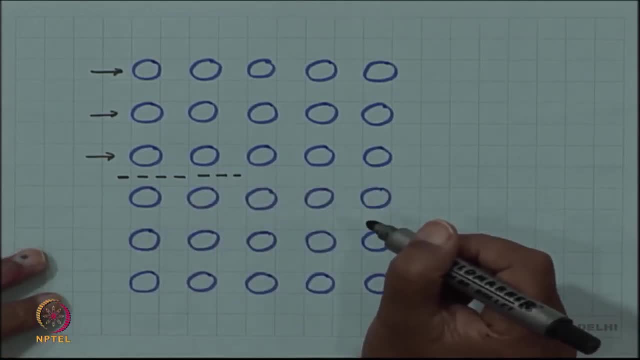 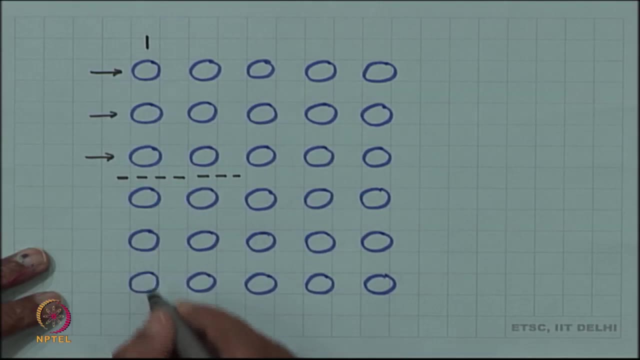 the cut Only up to the second plane. then what will happen? and I am pushing, let me label the planes. So I call this plane 1,, plane 2,, plane 3,, plane 4 and plane 5. I am labeling the vertical. 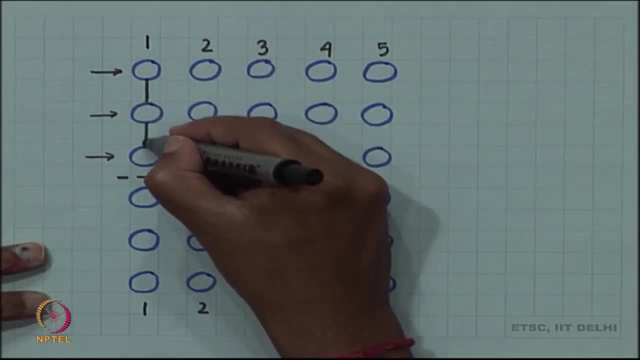 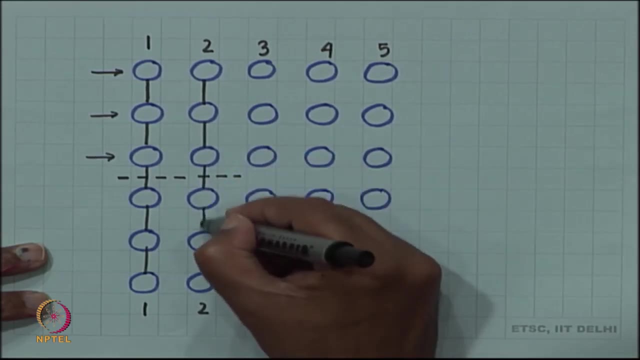 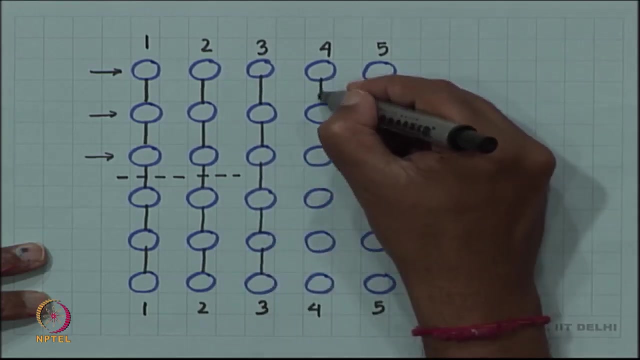 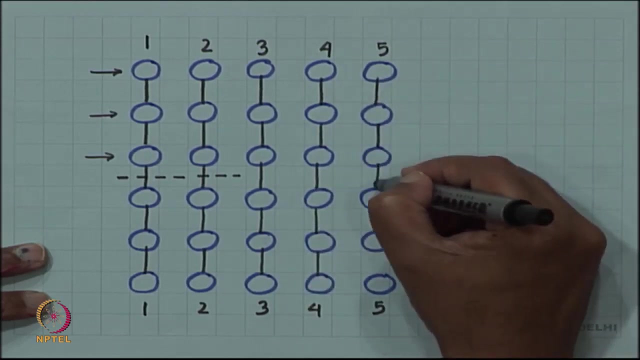 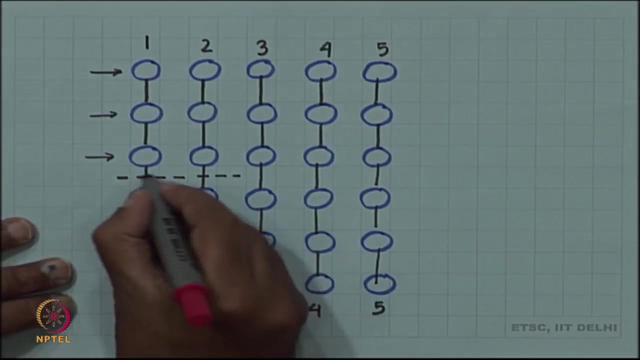 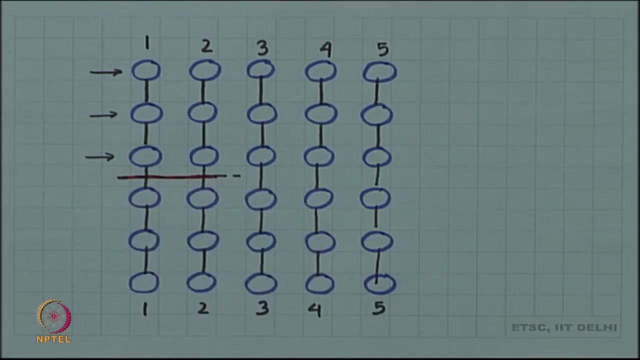 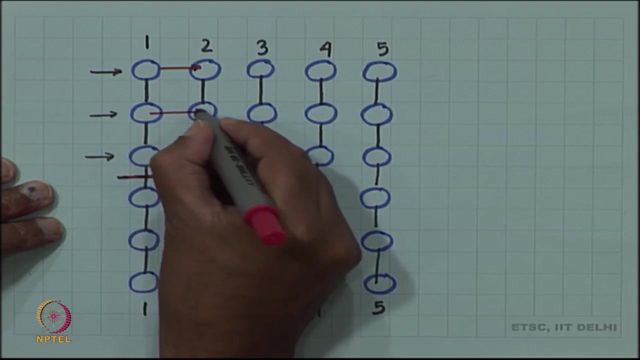 planes. think of these as a vertical planes. So I have these vertical planes and I have cut these bonds here. I have cut these bonds and trying to slide the crystal in a way such that the first plane shifts to the position of 2, to the second plane. 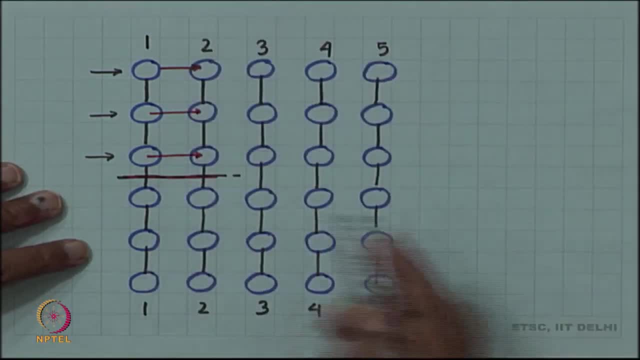 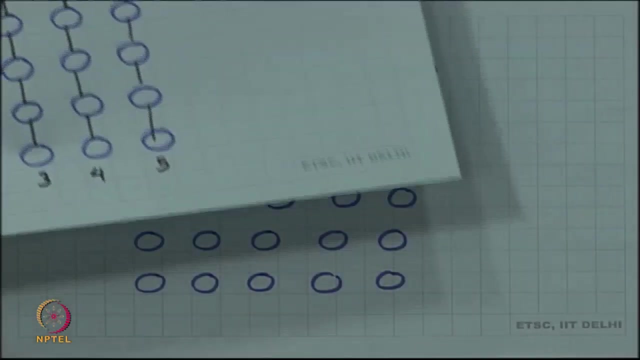 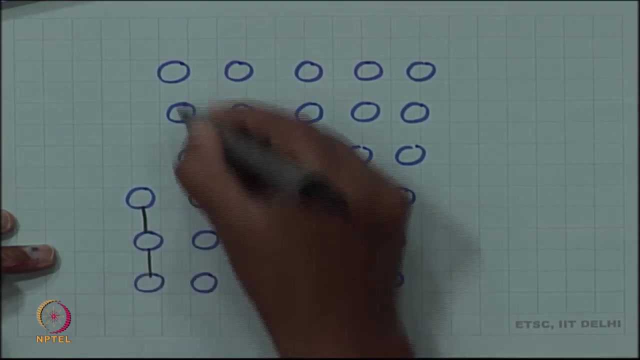 So second plane has to move to accommodate the first plane, but it cannot join the third plane because I have not cut any further bonds there. So what will be the configuration which will be generated by this process? So you have already seen in your study of dislocation that then, since you have the first, 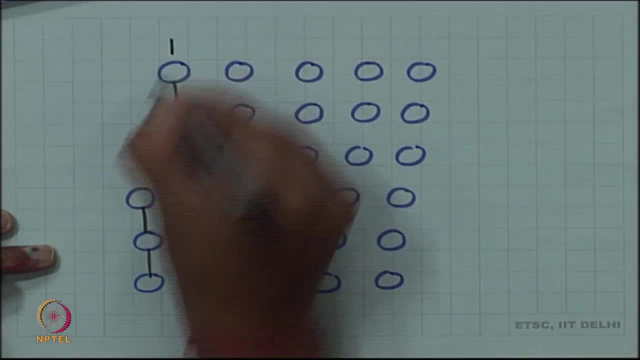 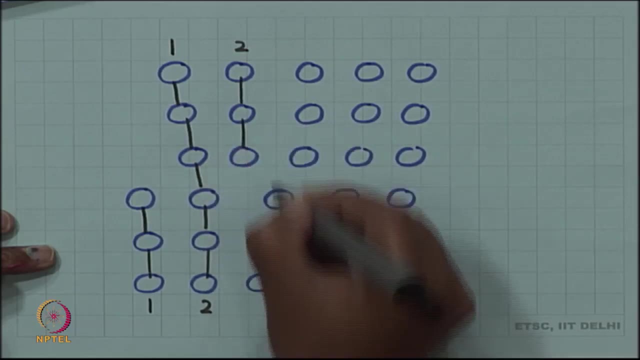 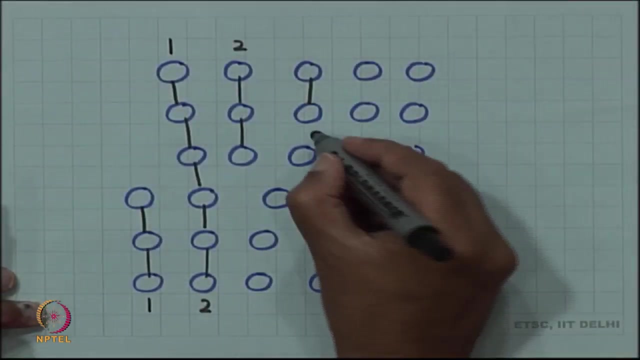 plane joining with the second plane. the first plane from the top is joining the second plane from the bottom, but the second plane from the top is not able to join the third plane because third plane is continuous. Remember, I have not cut the bond there, so the third plane just deforms to accommodate. 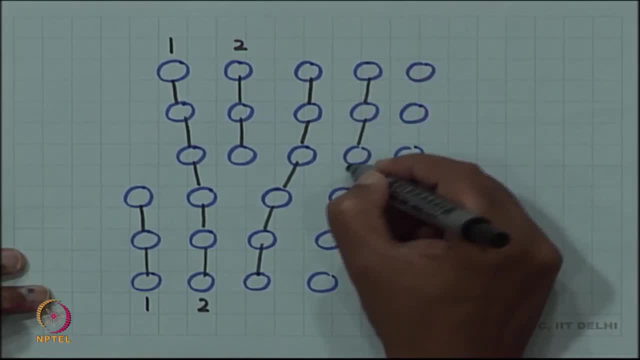 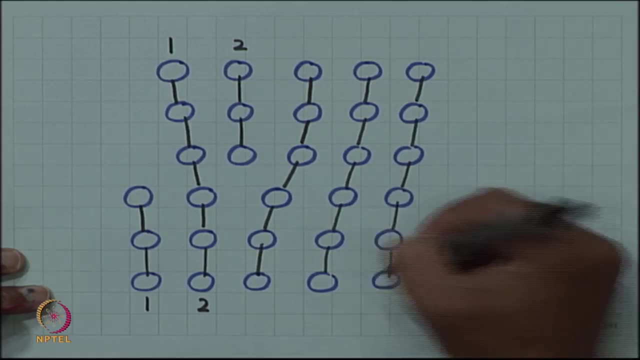 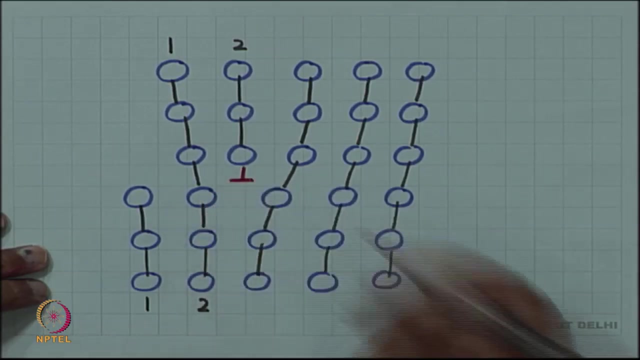 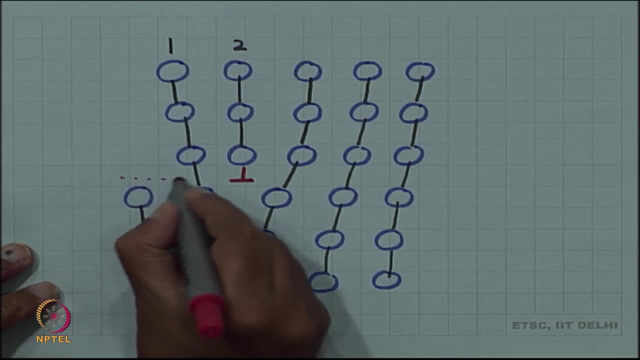 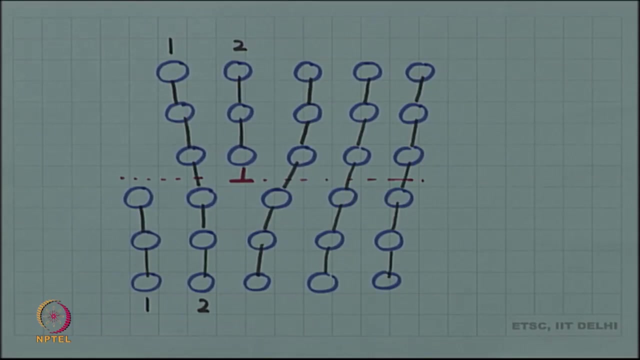 the second half plane from top. So we have created a half plane and we have seen that there is a dislocation which has appeared now. so I am using the symbol of dislocation- edge dislocation, which we have introduced In our defect chapters. now, why should this process be easier than deforming like a rigid? 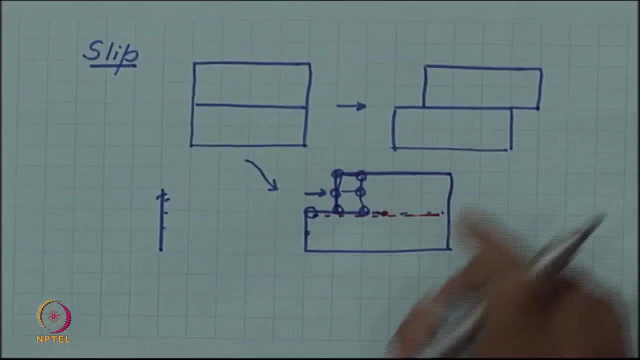 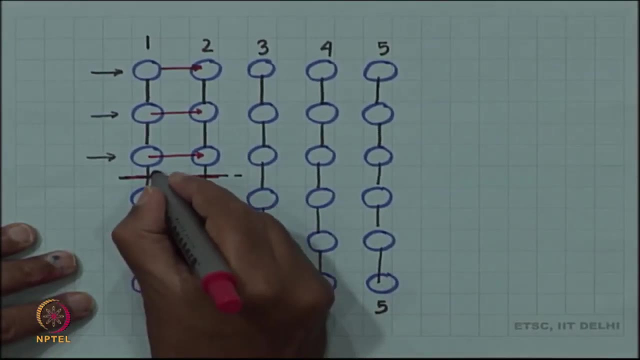 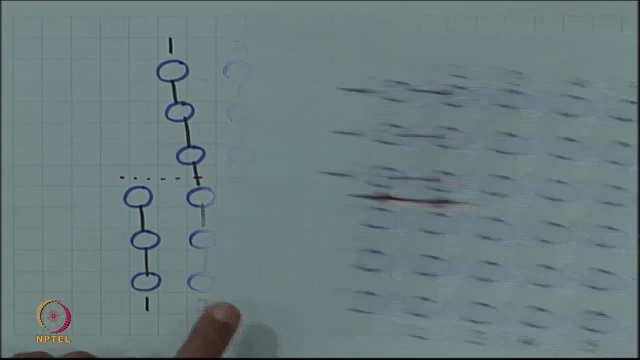 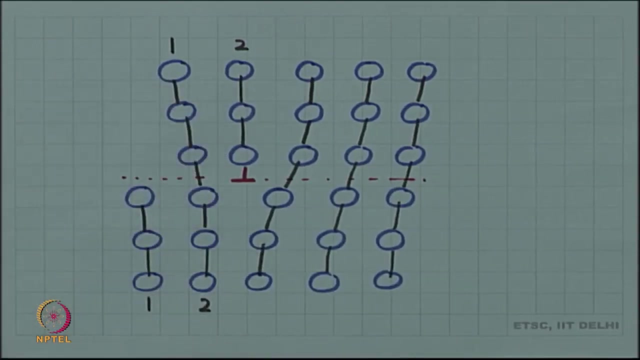 body deforming like this, like a rigid body over the entire plane. You can see that here we have to cut only the two bonds To introduce this step. I have cut only these two bonds and then I am able to deform and create this extra half plane. 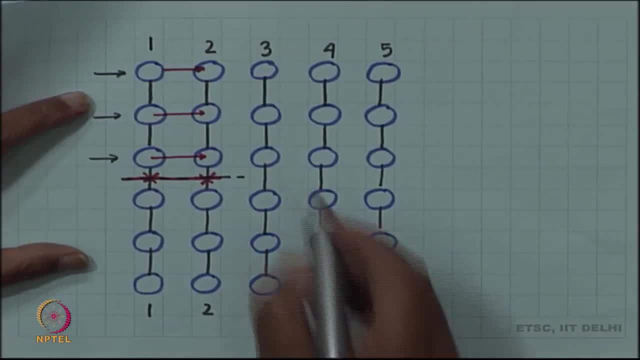 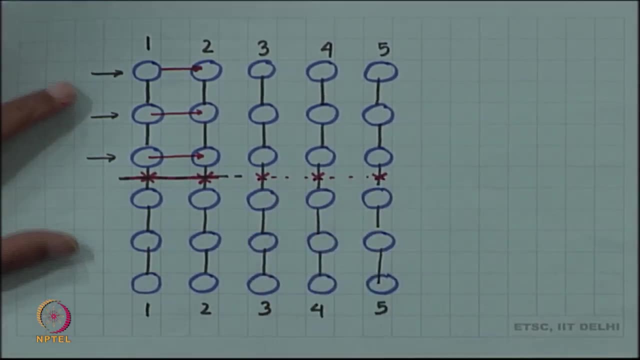 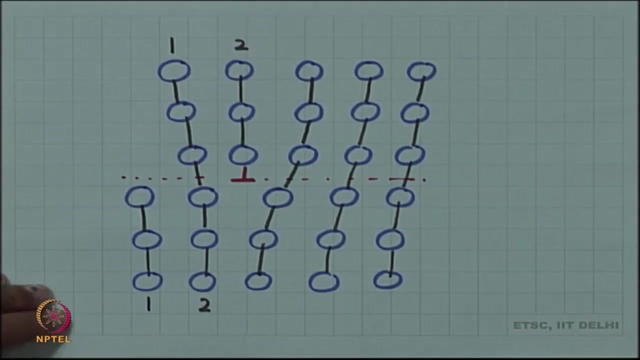 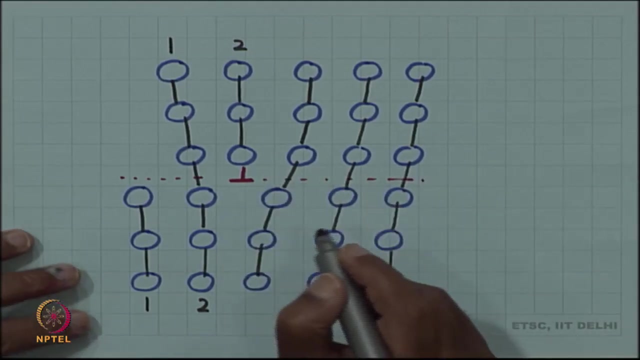 If I wanted a complete step, then I will have to cut all these bonds in one go, so that will require a higher energy and correspondingly a higher stress to achieve it. So in this case, for each unit step from now onwards, I have to cut only one set of bonds. 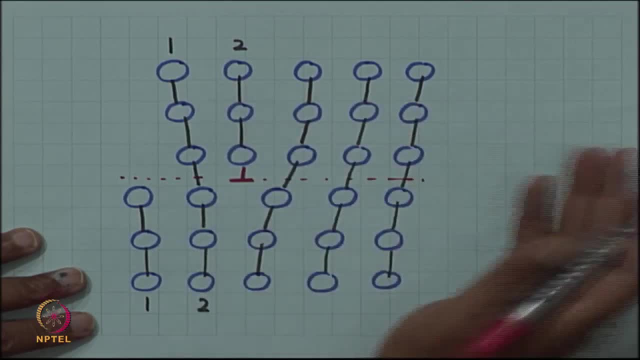 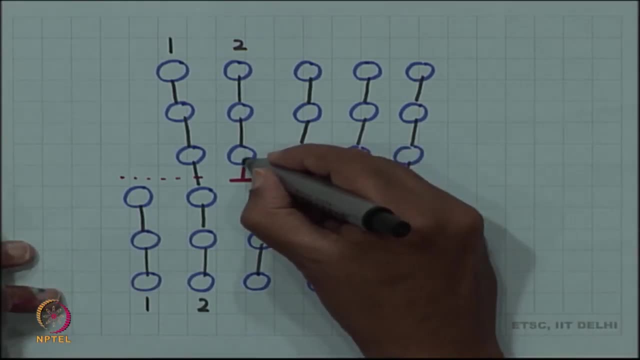 So what I will do now to create further deformation, I will just cut this bond such that this bond now rejoins here. so I have now the second plane joining with the third plane from the bottom. This is exactly where it is, where it relates. 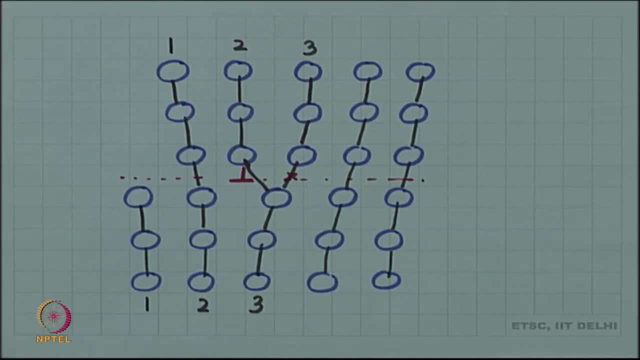 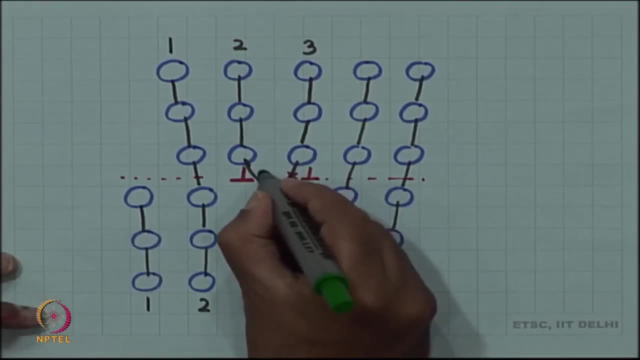 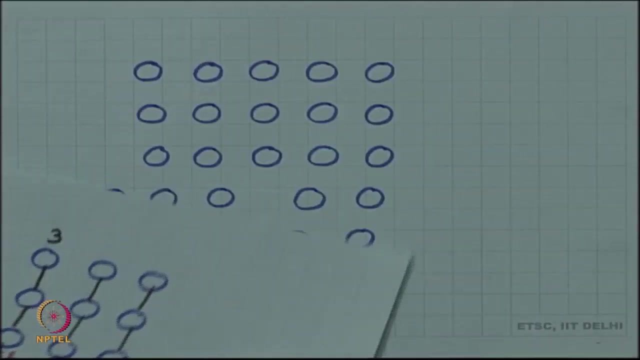 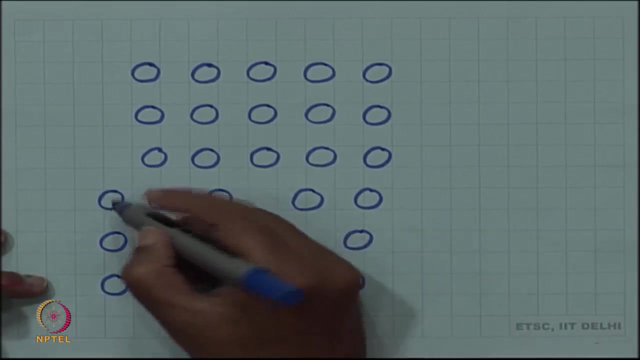 Whereas the third upper plane is hanging. so the dislocation line, dislocation line moves one step. this is what we show in the next picture. So now dislocation line has moved one further step. Ok, Classic, Ok. 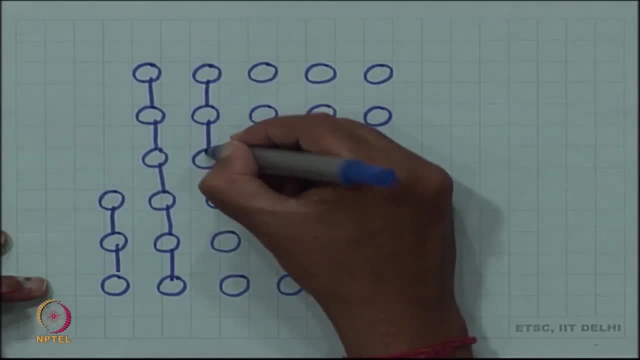 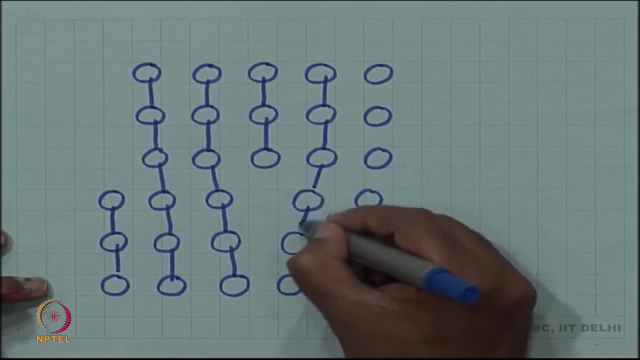 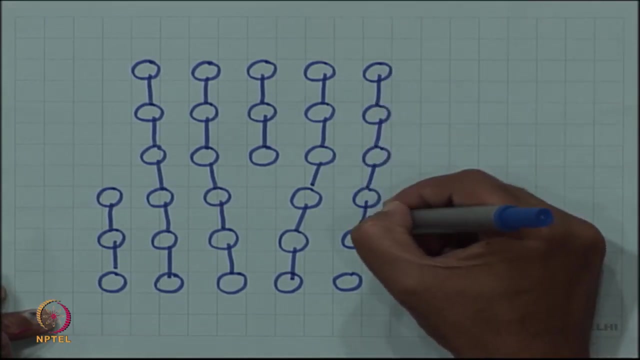 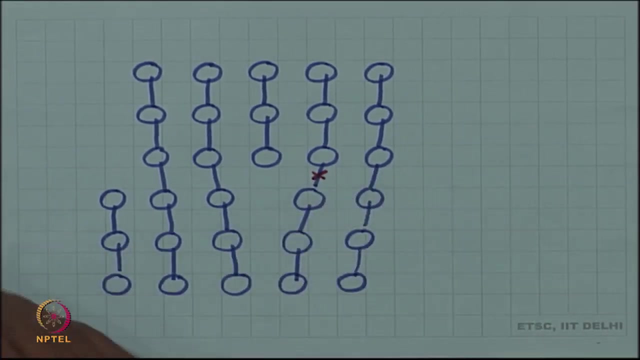 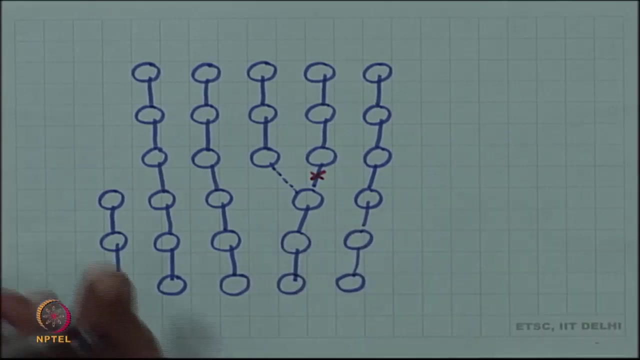 So it has come to the third plane from the top now. so, gradually, if we keep moving it this way each time, now for yet another step, I have to just break this bond and connect it this way, So it will go to the fourth plane instead. 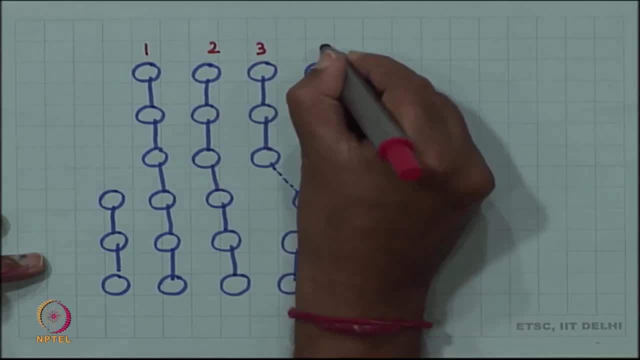 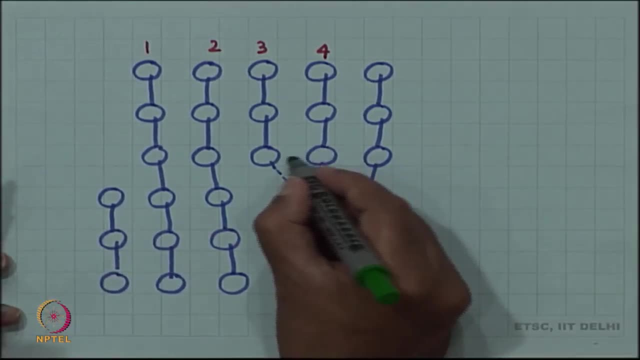 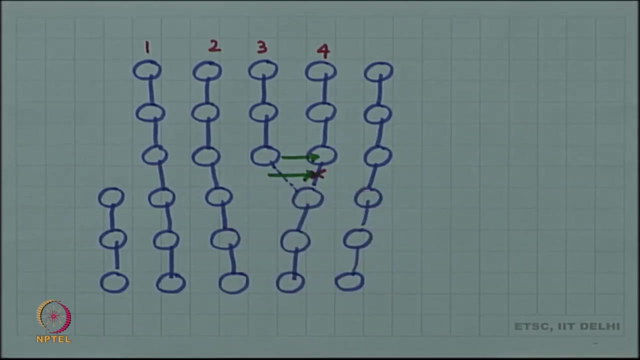 of currently 1,, 2,, 3 and it is on the fourth plane. it is in the third plane. So from third plane it will move to the fourth plane. the dislocation will move from here to here. So that is shown in this picture. it has now moved to the fourth plane. 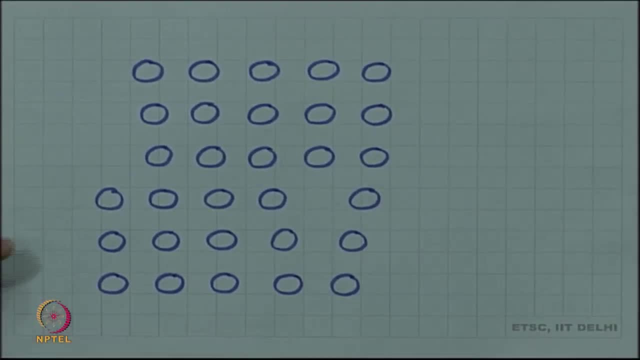 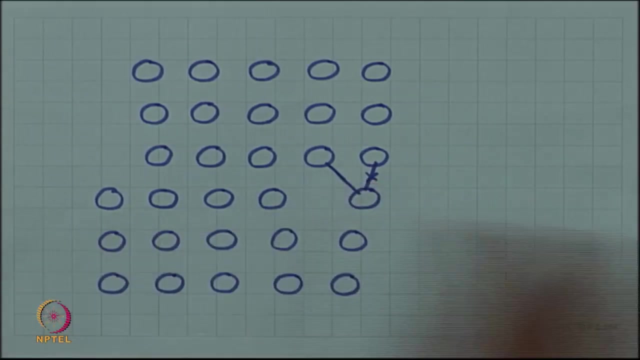 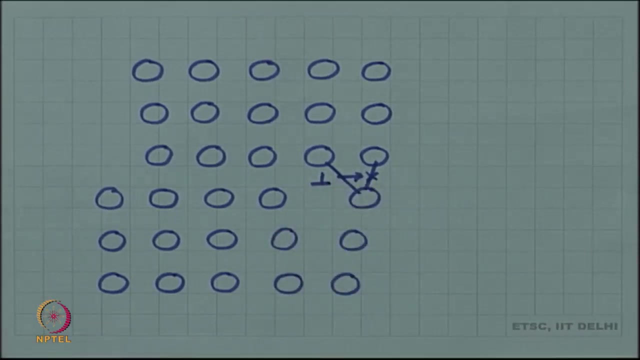 Now there is only one external plane left outside and once I break this bond and connect it here, then there will be this half plane moving out, the dislocation will be moving out of the crystal and we will create a unit step in the crystal. So this is the final. 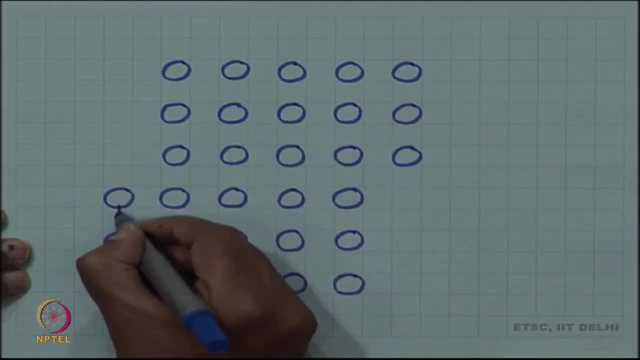 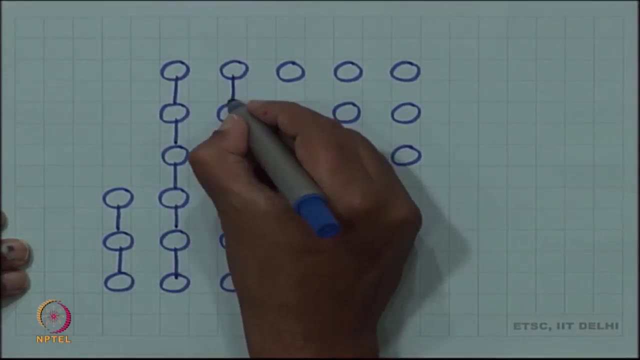 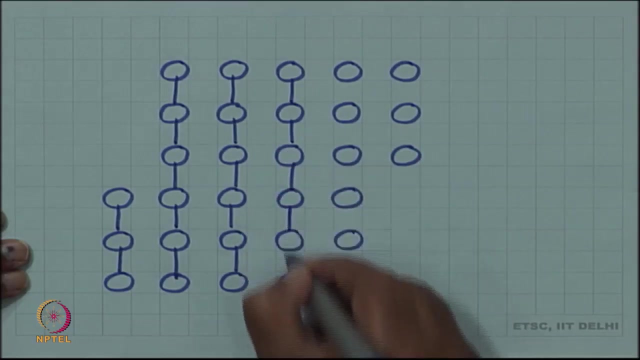 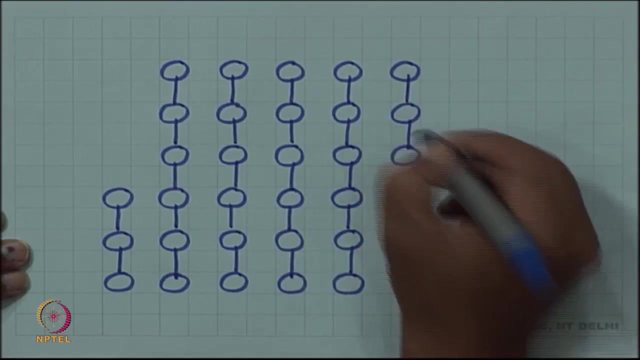 arrangement where the extra half plane has now come out of the crystal. So you can see that final deformation. in the end we have achieved the same configuration which we would have obtained by a complete single step. rigid body deformation of the upper half plane.